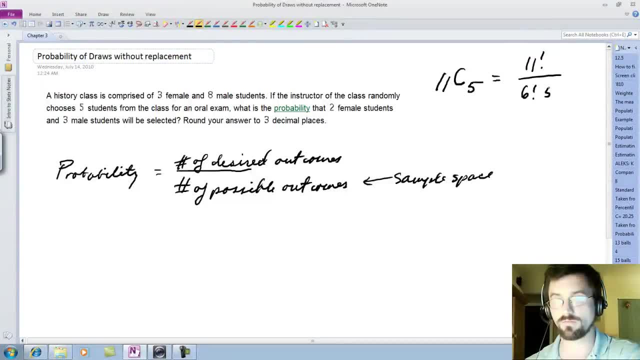 11 divided by 6, 5.. Remember: this number here is always 11 minus 5, because it's n minus r. Okay, if you forget the formula here, I'll show it to you real quick And then we'll do it again. 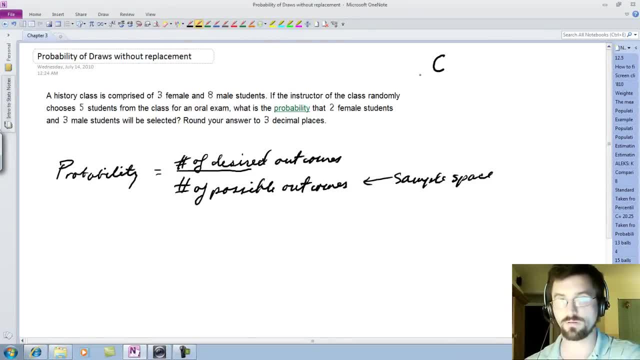 So the formula for combinations, When we're choosing r out of n, it is n factorial divided by r. oh whoops, n minus r in parenthesis. factorial times r factorial, And the rationale is: these guys figure out the number of ways that you can choose. And this one here takes out 11,, 5,, 4,, 5.. And the other one here takes out 8,, 5,, 4,, 5.. And the rational is: these guys figure out the number of ways that you can choose. 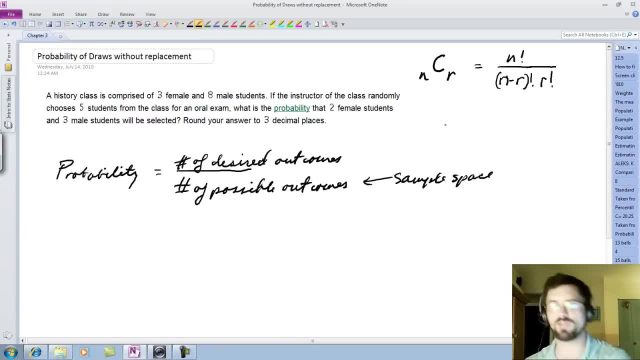 And this one here takes out 1, 6, 5, 4, 5.. all the repeats, but that's in a different video. anyways, you just need to know to use this and it's 11. choosing 5, it's going to be 11, factorial over 6. 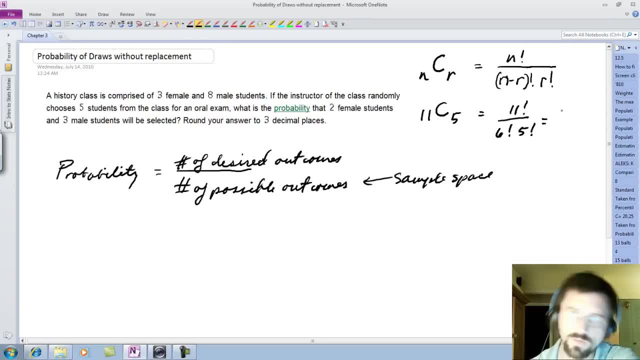 factorial times 5 factorial, which we know is going to be me. erase some of this. it's going to be what it's going to be: 11 times 10 times 9 times 8 times 7 times 6 factorial- over 6 factorial times 5 factorial. that kills that 5 factorial. 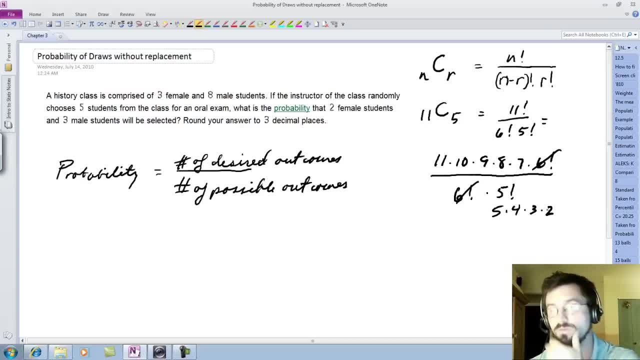 is 5 times 4 times 3 times 2. so 4 times 2 takes out the 8, 5 goes in 10, leaving 2. 2. 3 goes into 9, leaving 3. okay, so that is the denominator. it is 11 times 2. 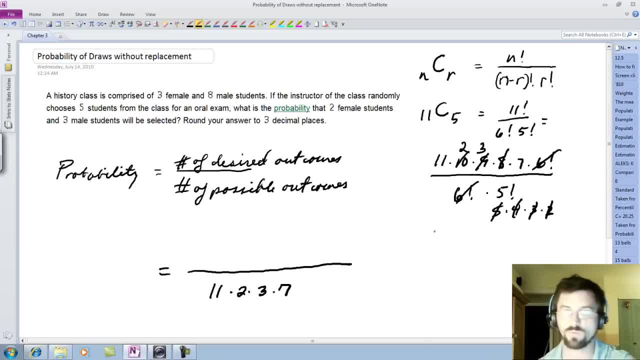 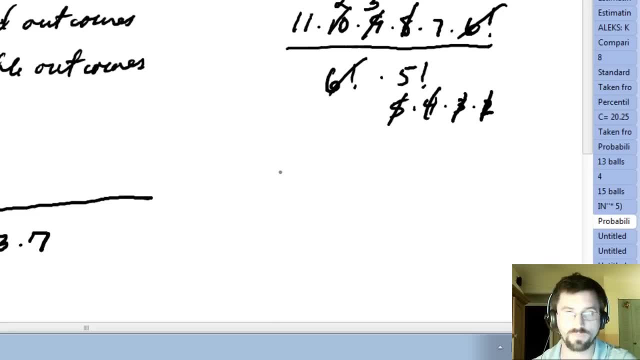 times 3 times 7, and you don't have to calculate that because we'll have more cancellation in the numerator we have. we want to choose 2 females out of a possible 3. so 3 choose 2. that's for the females. for the males, we have 8 mils and we're going 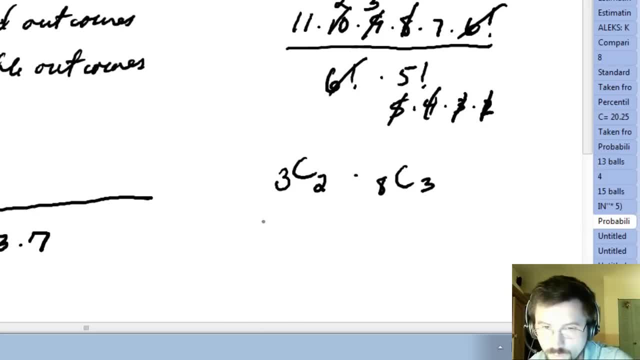 to choose 3. so, using the formula, we have 3 factorial over 1 factorial times 2 factorial, and hopefully you'll figure out after a while that whenever these differ by 1, the answer is n. okay, so that comes out to 3. and then what do we have? 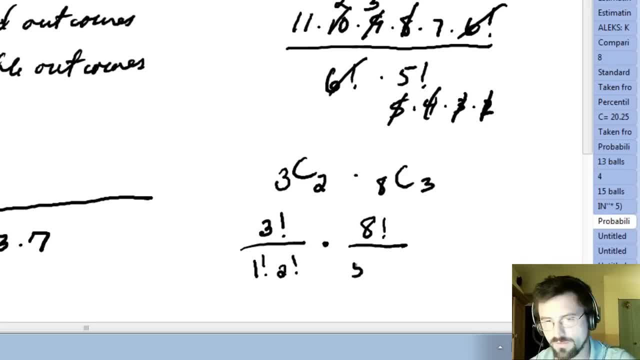 over here we have 8 factorial, 6 capital impacted, 8 and 5 factorial over 16 times 6 factorial, that's 5 factorial of those 3 factorial. now you could go like this: and then 2 goes into- well, you can't show to- goes into 8, because you gotta write this out. so 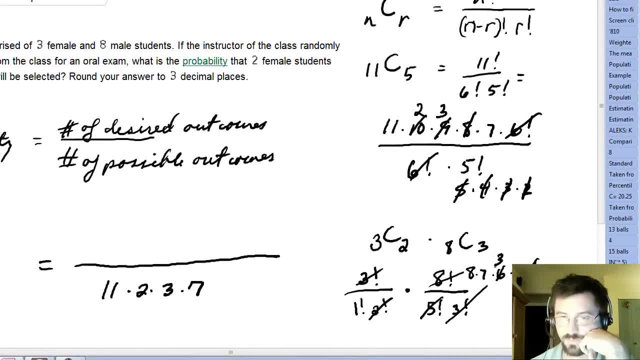 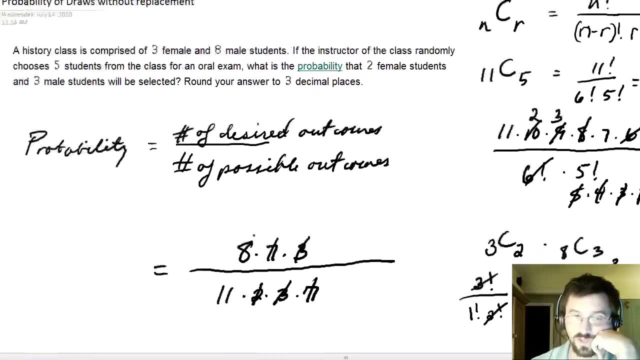 we'll rewrite this as 8 times 7 times 6 times 5. factorial 5 takes out 5 and then 2 goes into 63 times the 3 and the 3 go away, the 7 and the 7 and I'm left with oh, and the 2 goes into the 8. 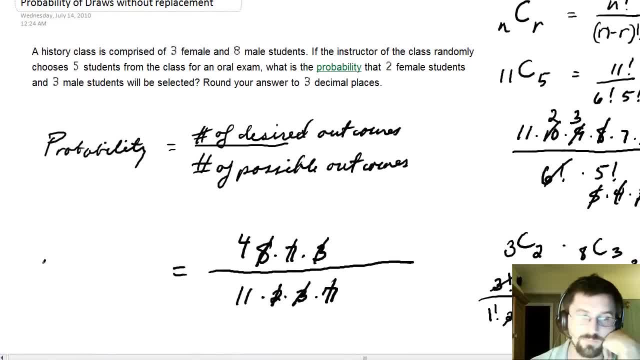 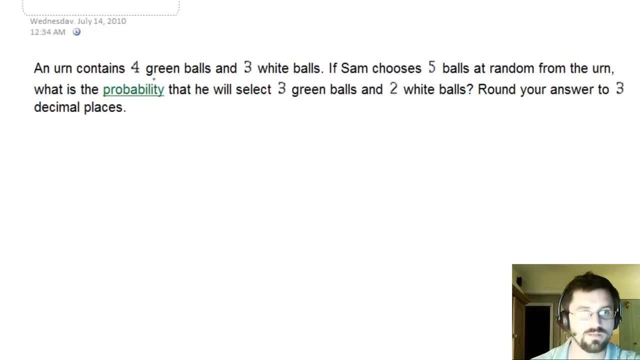 4 times. so I'm left with 4 over 11, and that is my probability of what is it? 2 females and 3 males. now let's do another one and earn. contains 4 green and 3 white, so we have 7 balls, and how many are we going to choose? 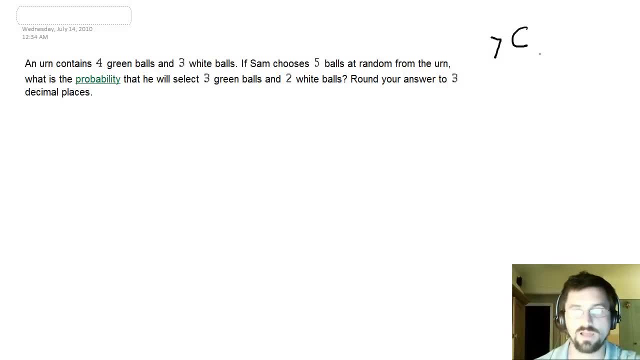 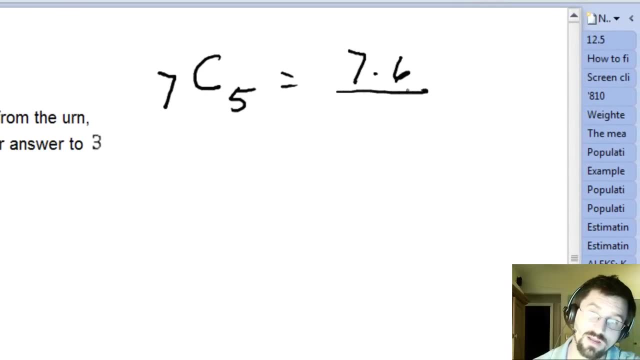 5 balls at random. so 7, choose 5, so it's it's going to be 7 times 6, divided by 2, and you can do the math on that to confirm that it's 21,. now use the formula and make sure you understand. 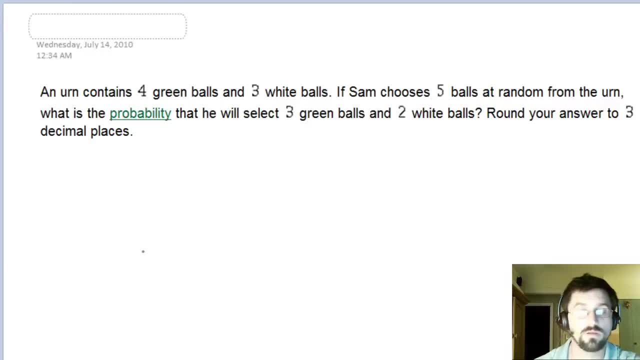 how I got that. so that will be the sample space, the number of possible outcomes, and now we need to figure out the favorable ones. we want to know what is the probability that, choosing 5,, he will select 3 green and 2 white. 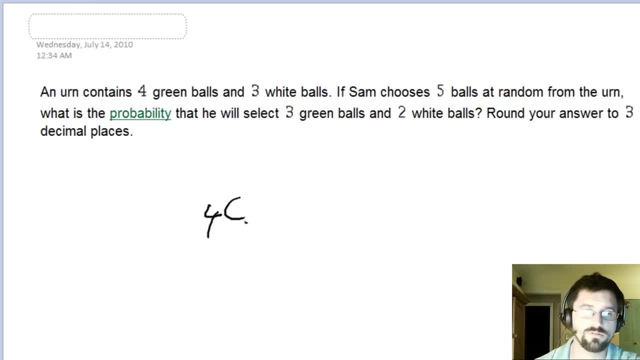 so 3 green out of 4, so that's 4 choose 3 times, and then 3 choose 2. so this is for the green, this is for the white, and I just told you a second ago when these guys differ by 1. 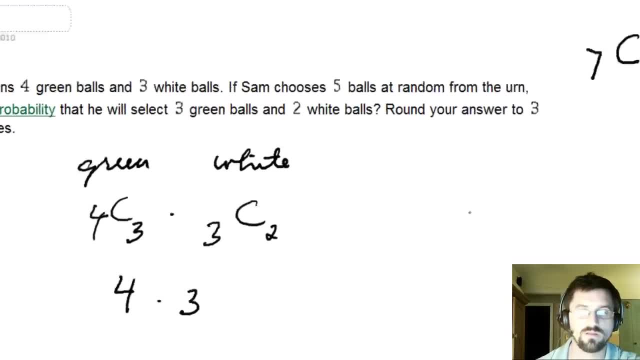 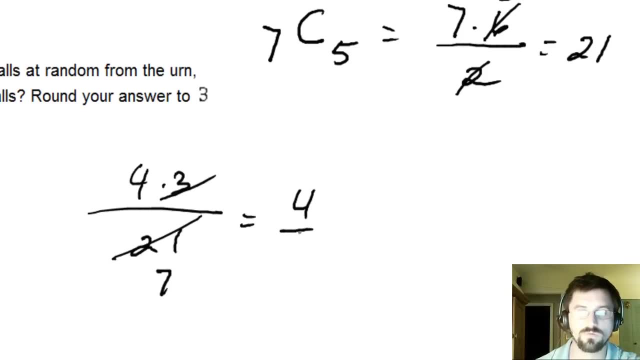 the answer is always n, so it's 4, it's 3, so we have 4 times 3 over 21, which goes in 7, so our answer is 4 over 7. it's the probability of 3 green and 2 white. 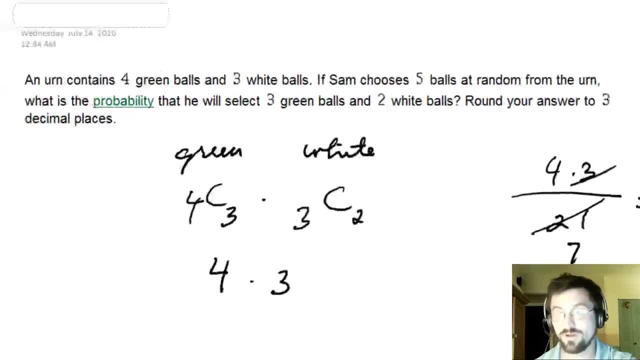 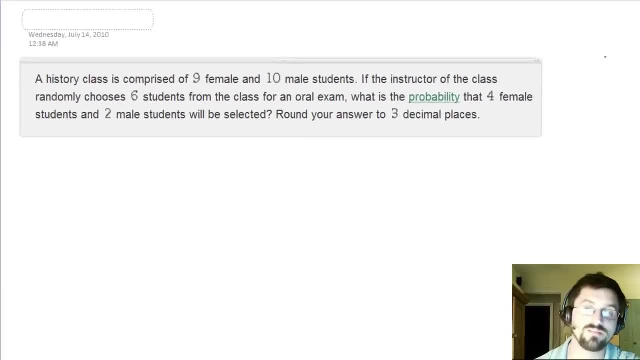 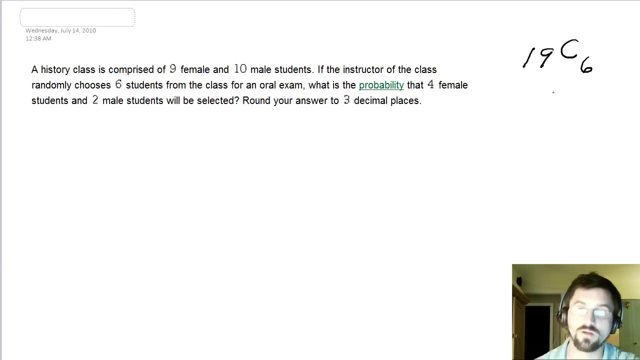 alright, hopefully you're getting the hang of this. let's do another one. history class 9 females, 10 males. so our sample space is 19 and we're choosing 6, so it's 19. choose 6, so it's going to be. 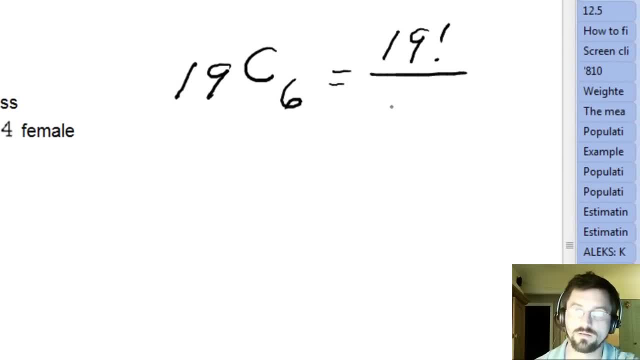 19 factorial divided by 13 factorial times 6 factorial. so that's going to be 19 times 18 times 17 times 16 times 15 times 14, the 13 factorial that will come after that will cancel with the 13 factorial. 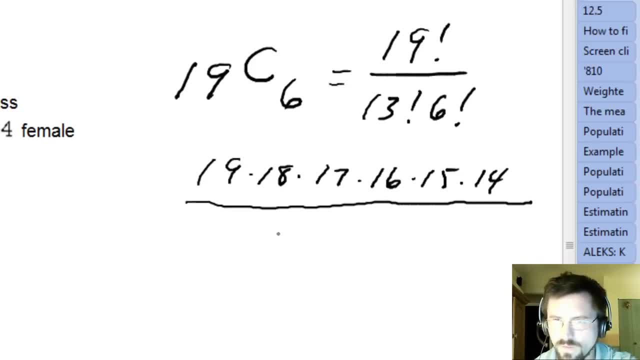 on the bottom. and so then we have we have 6 times 5 times 4 times 3 times 2. alright, 4 times 3 is 12. nope, what do I want? let's do 3 and 6. take out the 18. 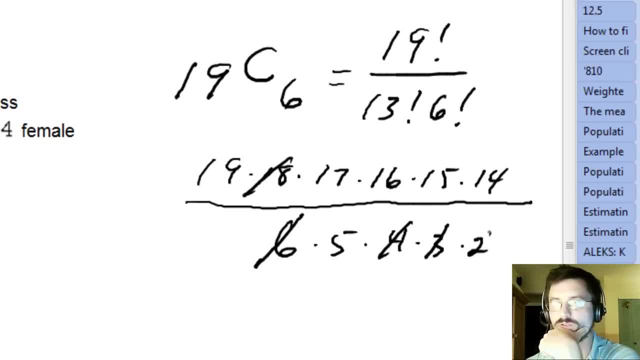 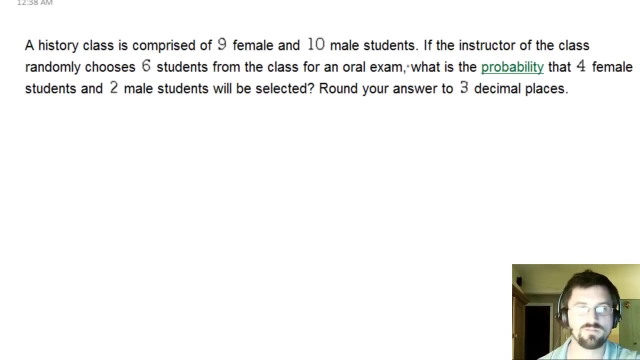 4 and 2 go into there and leave a 2. 5 goes into 15 three times. so that's my denominator. now they want to know what is the probability that 4 female students are chosen. so 4 out of 9 are chosen and 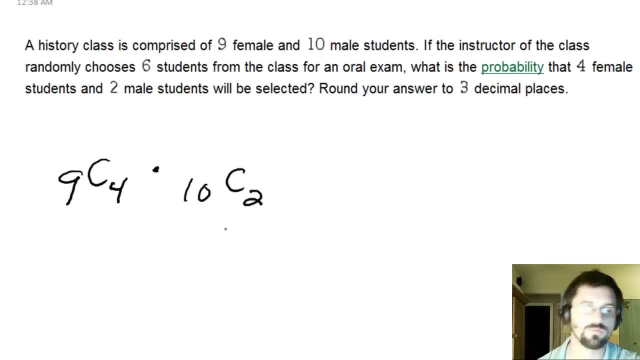 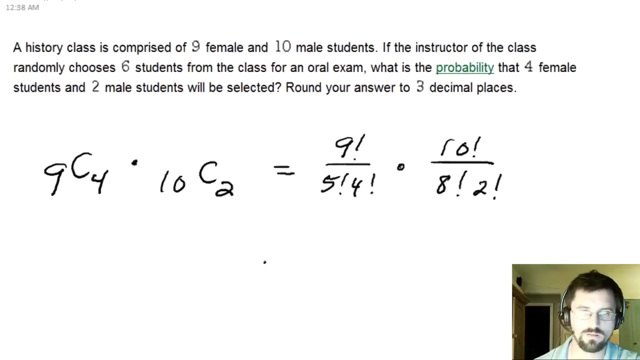 2 males, 2 males out of 10. so 10 choose 2. so our numerator is going to be 9. choose 4 is going to be 9 over 5, 4 times 10 over 8, and then two, and this one's pretty easy. 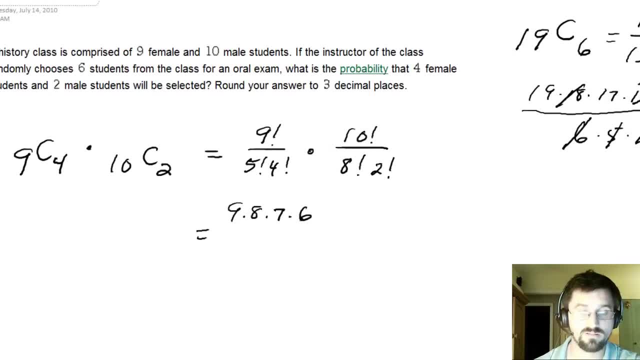 it's gonna be 9 times 8 times 7 times 6 over 4 times 3 times 2 times 10 times 9 over 2. take a moment and confirm that again when I'm actually here in my department. I am going to opt for it.